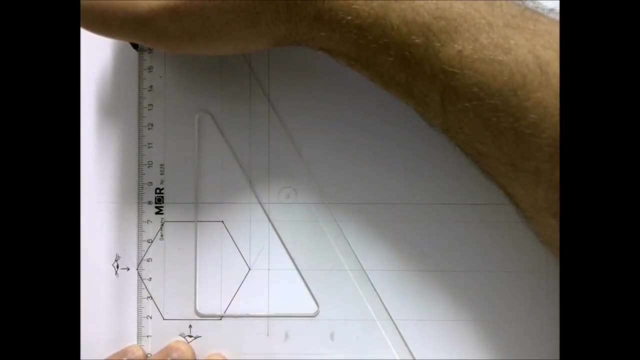 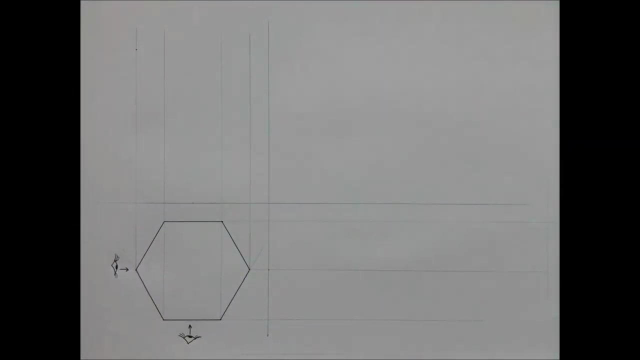 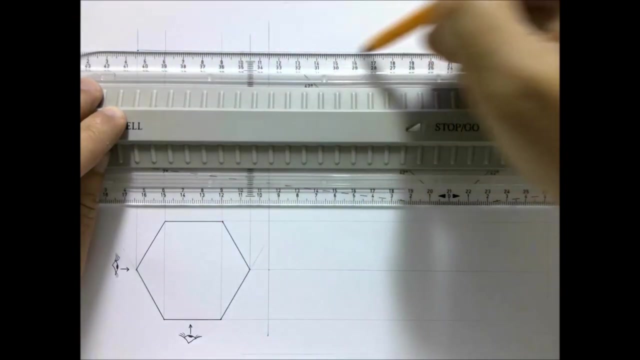 millimeters high. okay, so there's my 80 millimeter mark, in this case over here. i'm going to make it a pyramid, so i'm going to project that bit of information right across. remember, we're dealing with two two-dimensional shapes. so my top view, i would have a length and a width. 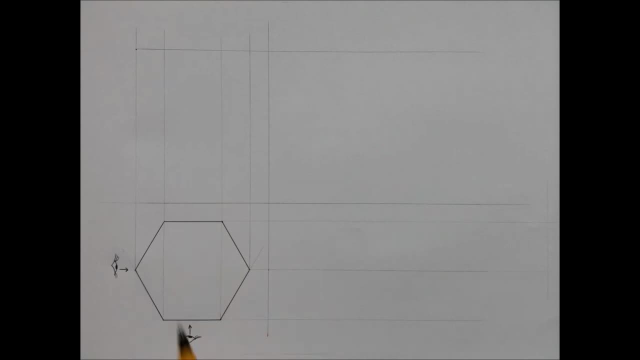 in my front view, i'd have a heart and a length, and in my left side view, i would typically see a width and a heart, obviously that heart being projected across to it, and then this width over here being projected up on my 45 degree line, because i'm only going to be projecting it all the way down, all the way up to the axes at this. 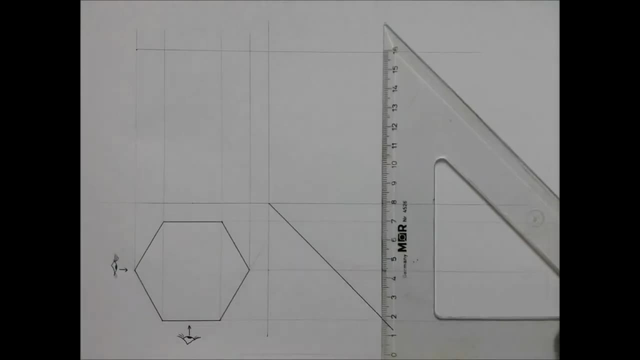 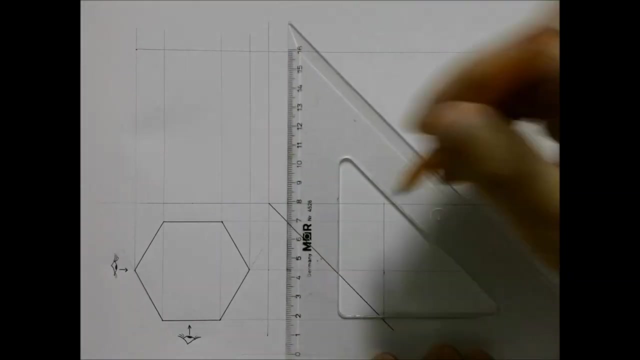 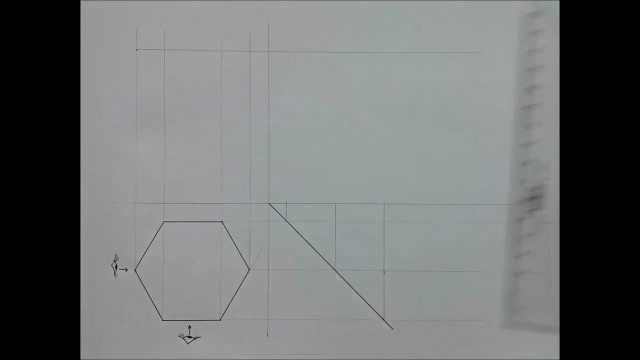 stage over here i can see how far or how much of my axes are touching the ground. see this, you can see in the top here, even if we have big activity around it. we have all this background here. we see it all there, and now you can go ahead. 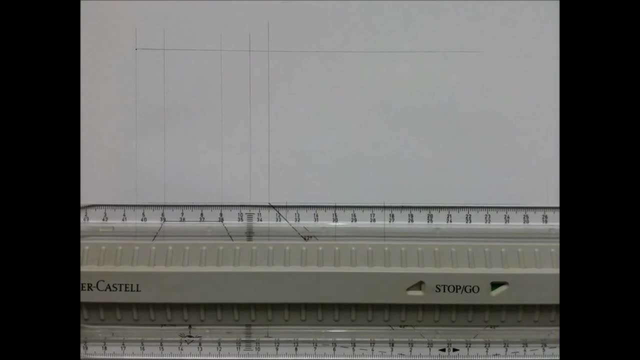 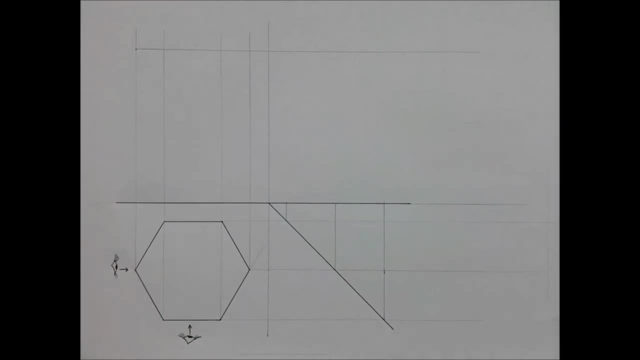 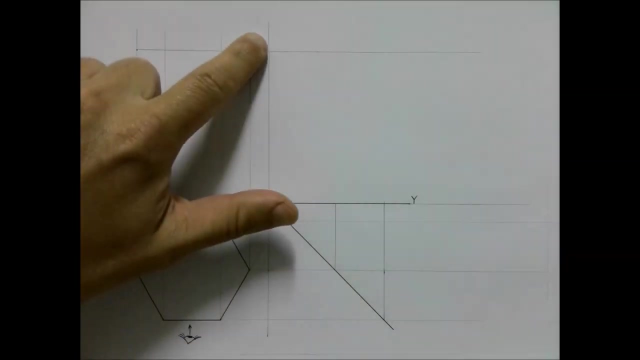 and present it schools need. so I can go ahead and then draw my axis. I'm gonna do it in freehand but you will have to go and label it between four millimeter guidelines we need. we read from left to right. therefore it will be X- Y and obviously X 1, Y 1. 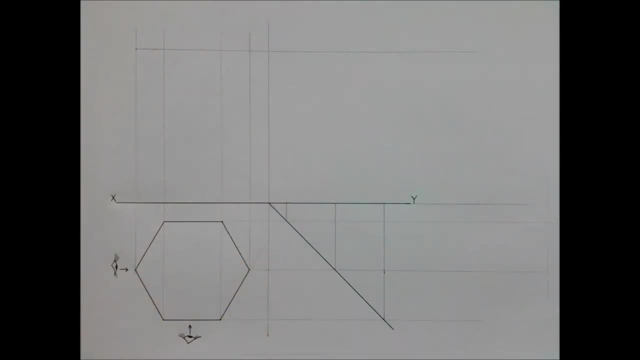 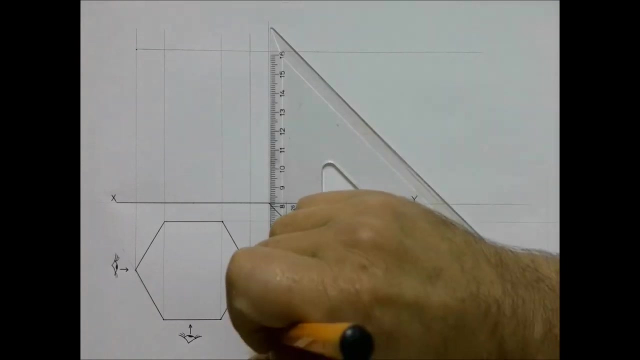 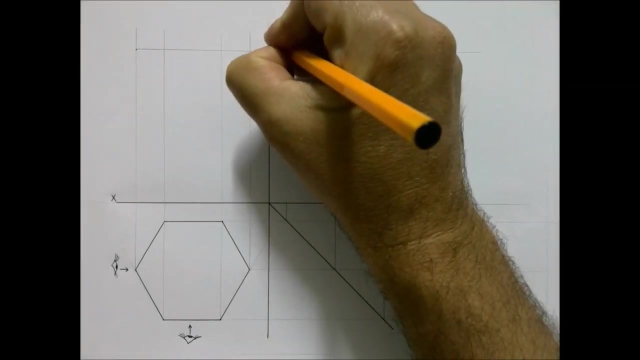 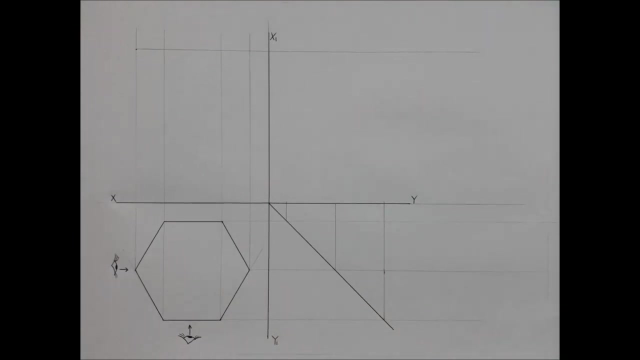 because we also read from top to bottom. okay in this case. okay, yeah, I can go ahead include my vertical access. all right, now I'm dealing with a pyramid, so obviously my hex engine, all my traditional suitable hexagons and locations, are made up of eight scrolling. 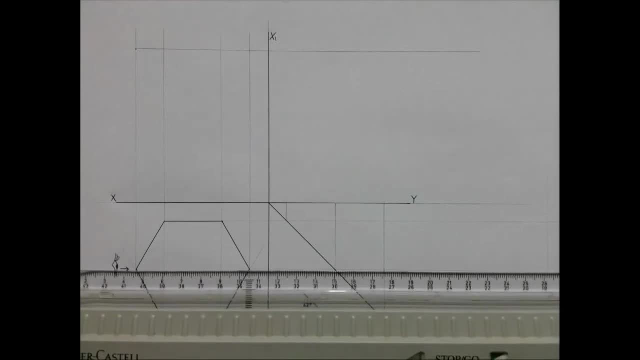 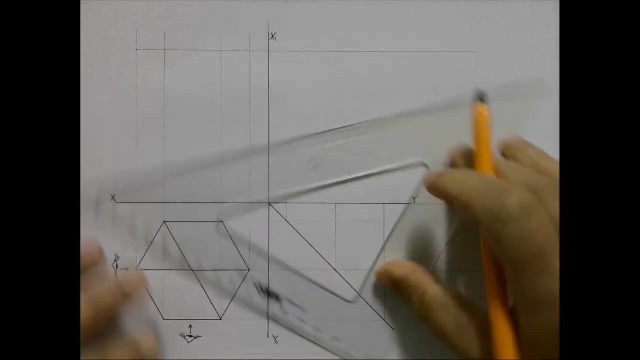 so obviously, my hexegons on myração- I made it all because I started the Elena top view- isn't going to be correct. If I may, I'm going to go ahead and connect all the opposite angles to one another, Providing that your hexagon is accurate. you'll be able. 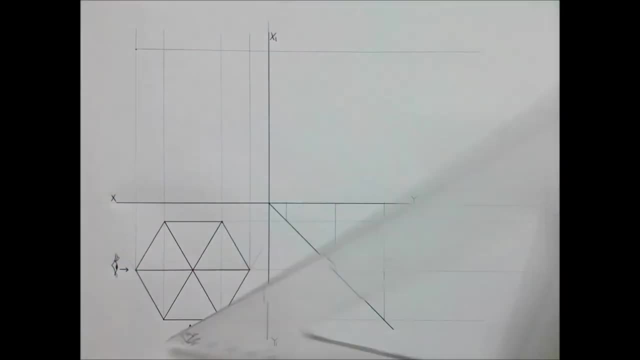 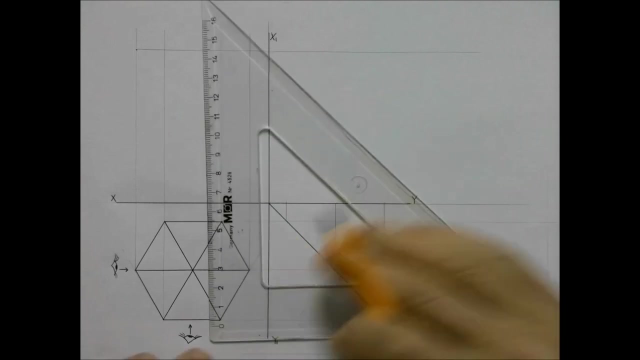 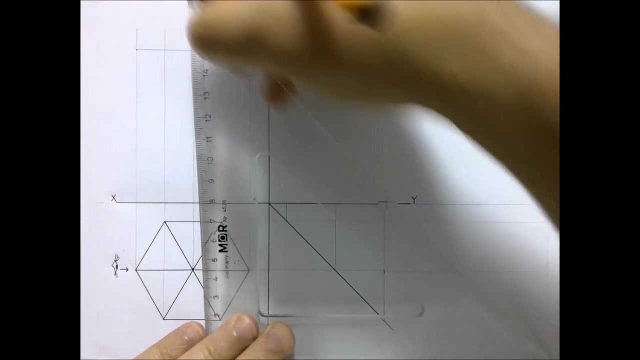 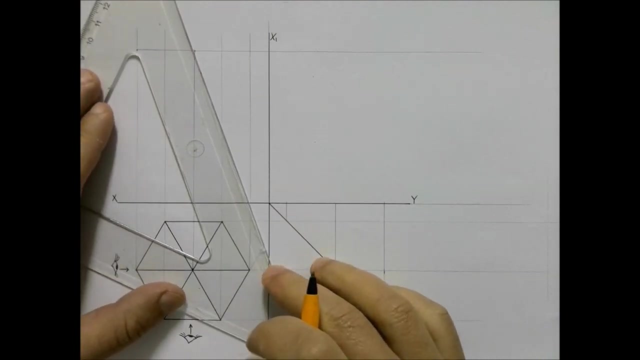 to have all your diagonal angles connect one another and provide you with the perfect centre. This is more information that I need to have to project up to my front view. Now I have the top of my pyramid. My front view will have the parameter drawings, parameter lines. 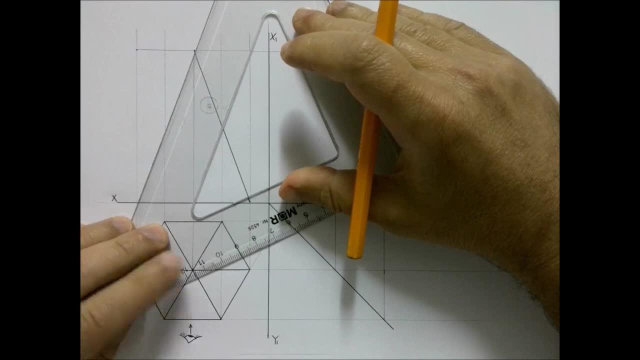 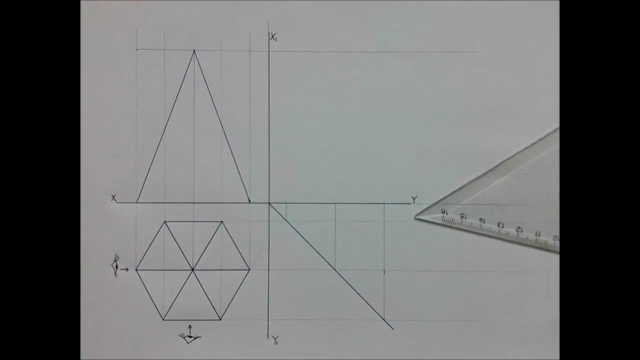 a profile, If you may, looking like. so, Obviously, when looking from this point of view, I'm going to see this surface over here, this surface over here and this surface over here. Anything behind this line, basically, will be in hidden detail or will not be seen. 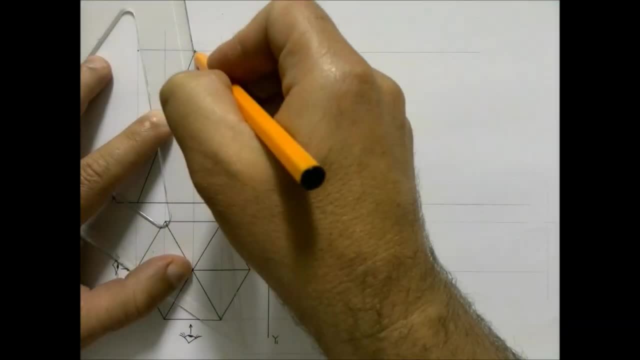 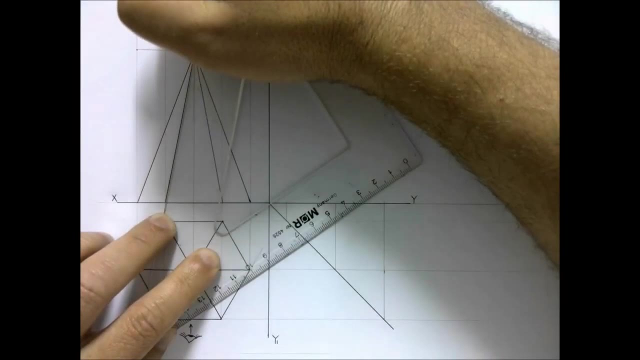 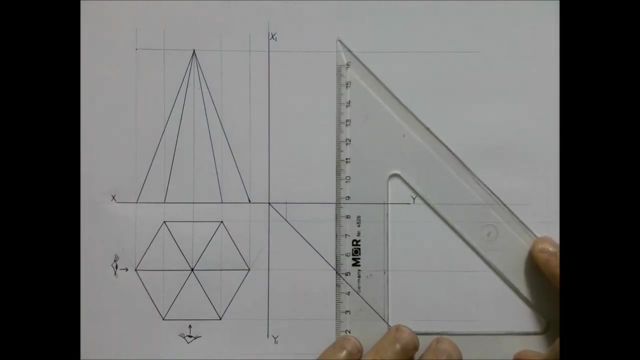 All right, I've got the heart. I can now go project the heart over there. Very, very important, You'll note yet again, from this side I'm going to be able to see where I'm going to see one, two, three surfaces, which proves correct when I look at my front view. 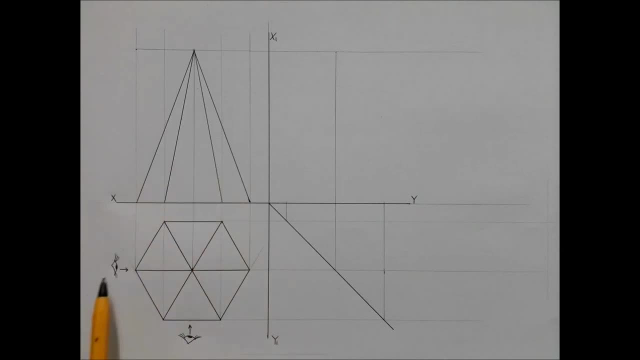 One, two, three surfaces. When I'm looking from this eyeball point of view, I'm going to see one, two surfaces, This surface and that surface. there will be flush. You won't be able to see these two surfaces, which means you'll only see these two surfaces In this. 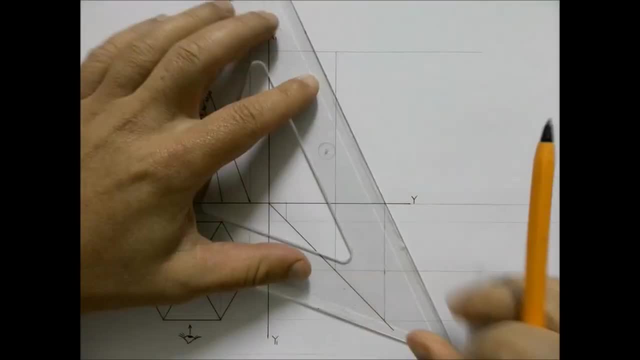 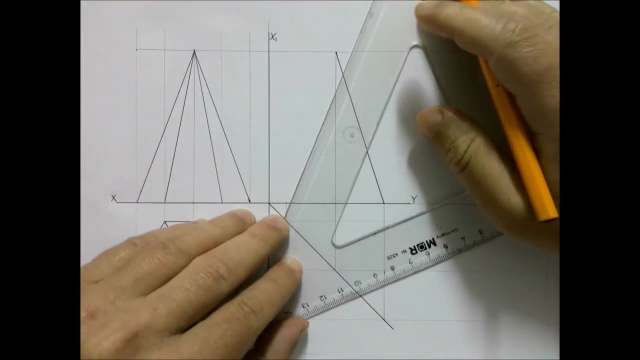 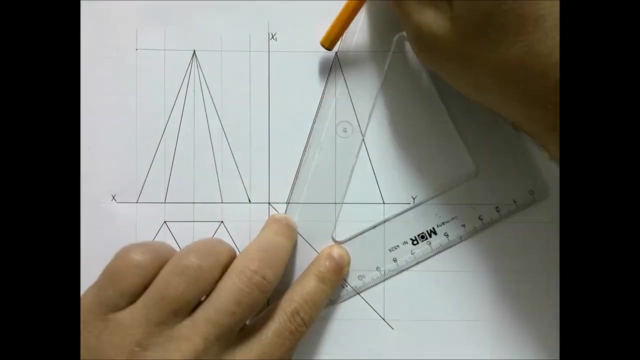 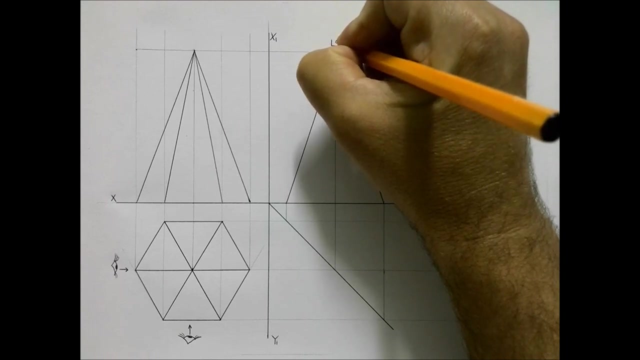 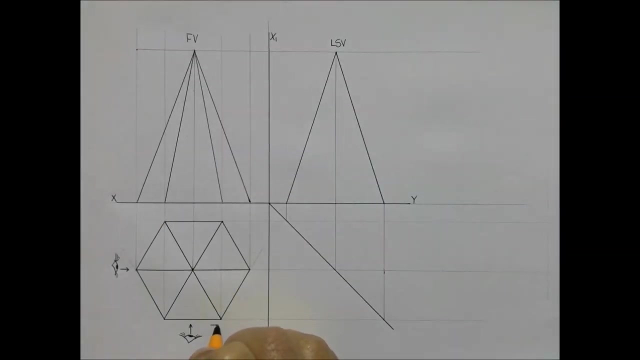